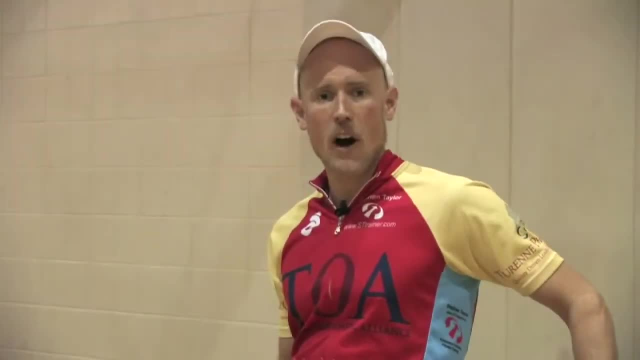 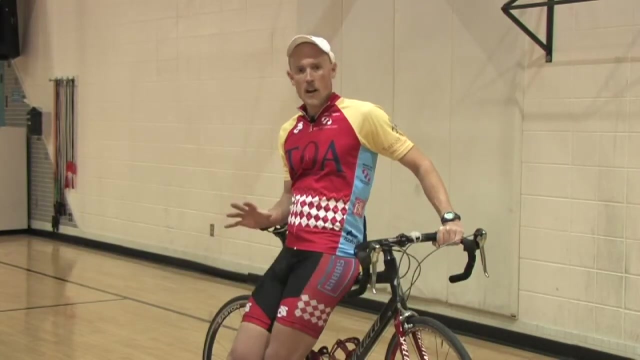 through a red light and do this in a safe manner without blocking normal vehicle traffic, then, as long as it's safe, use your judgment in those situations. Another question of safety is: where should one ride a bicycle on a roadway? There's a range of answers here. 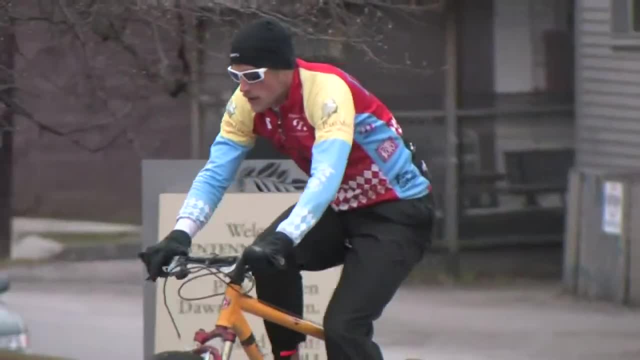 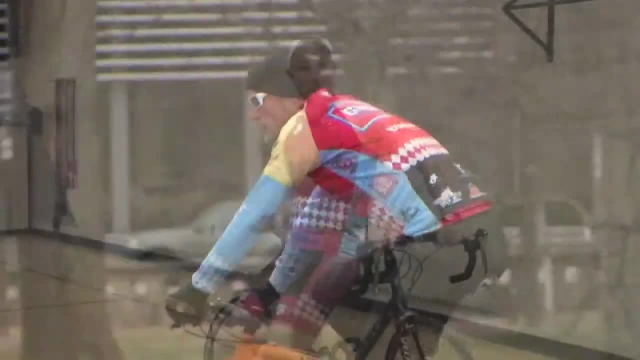 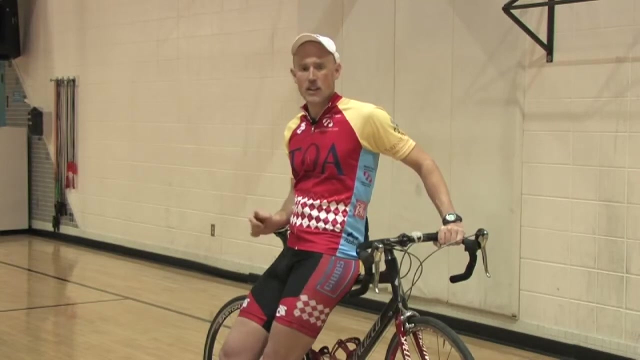 Generally, you want to ride on the right-hand side of the road as far as is safe and practical. In some situations, there may be little or no shoulder on the road or there may be hazards on the side of the road such as glass broken bottles. 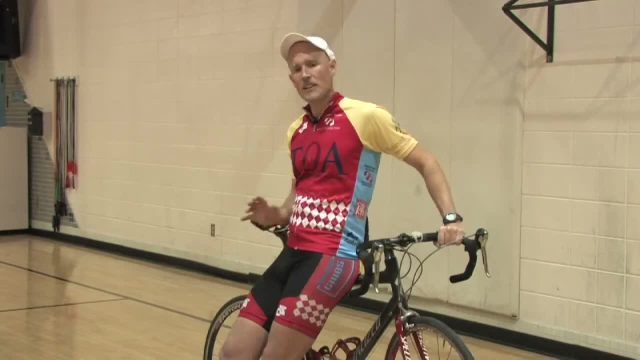 debris or a steep drop-off. In a situation like this, the safest place to ride is to actually move over two or three feet into the roadway. It's true, as a cyclist, that it is both your legal right and also your right to choose. 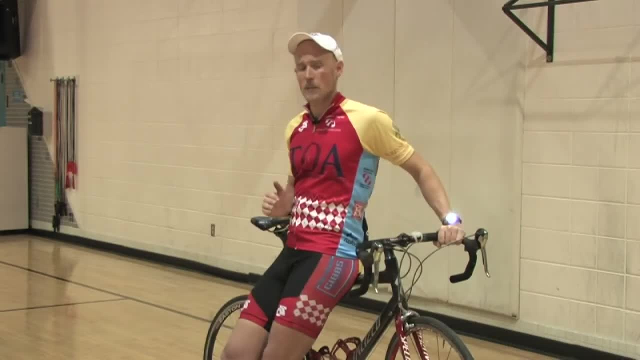 whether or not you want to ride on the right-hand side. So the safest strategy to sometimes position yourself in the lane of traffic as if you were another vehicle. This is very defensive riding and it's scary at first, but once you practice it a little bit. 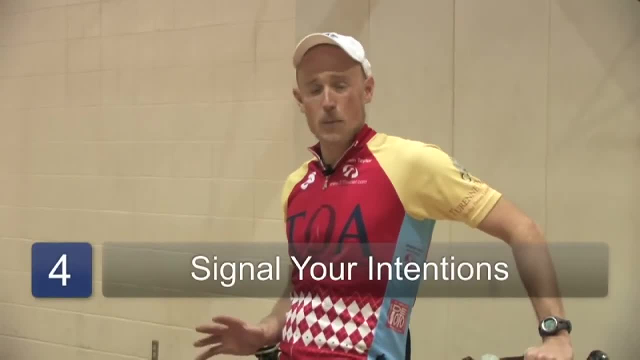 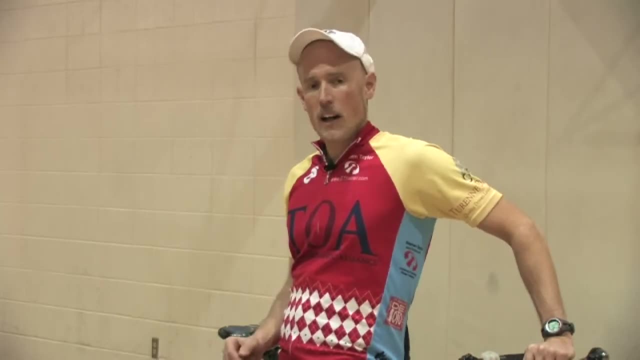 you'll feel more comfortable. Another safety consideration: a way to ride in a predictable manner is to be sure to signal your attentions. So if you're riding down the road, or if you're in traffic or on the right-hand edge of the road and you're going to turn, 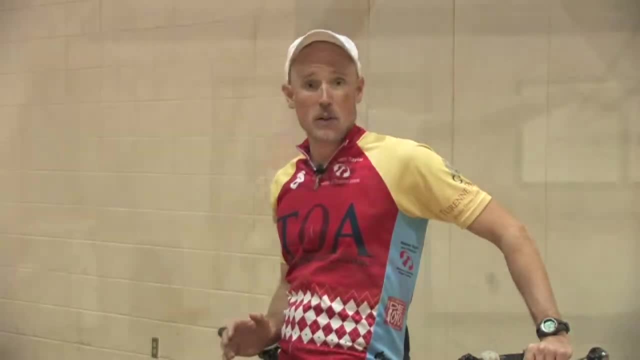 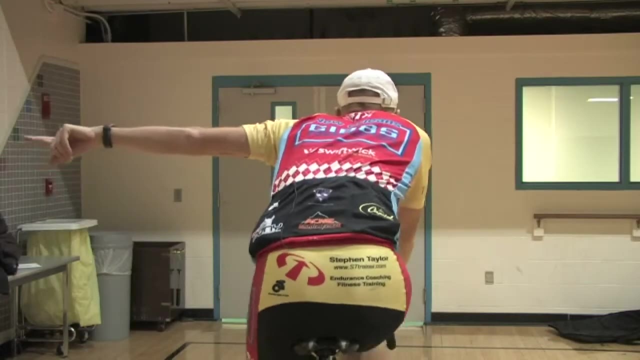 signal the direction you're turning. The way that I recommend you signal your turn is: point the direction you're going to go. If you're going to turn right, point with your right hand to the right. If you're turning left, do the same thing. 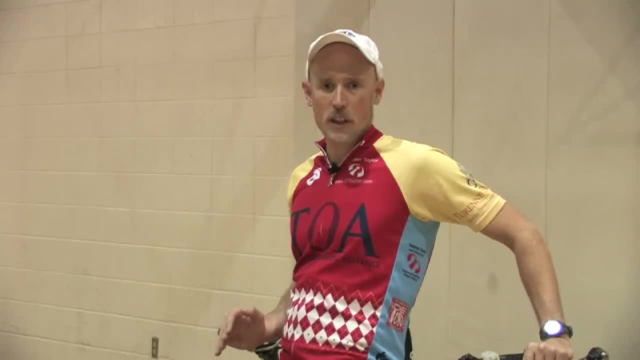 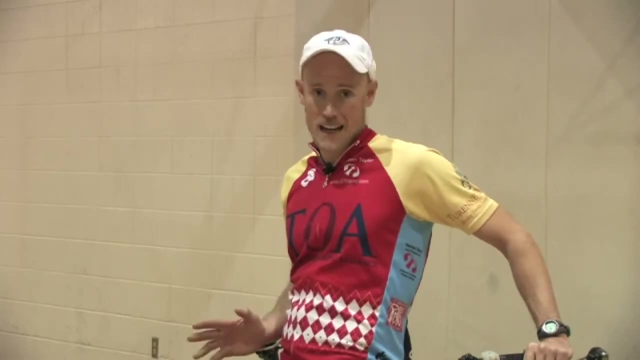 with your left-hand turn. I find that it's sometimes confusing and the younger generation does not know what it means to signal a right turn with your left hand. with the bent left arm You can also signal and gesture to automobile traffic and other cyclists that you're getting ready to slow down. 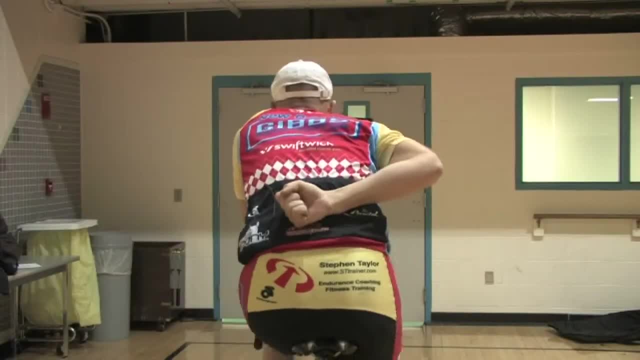 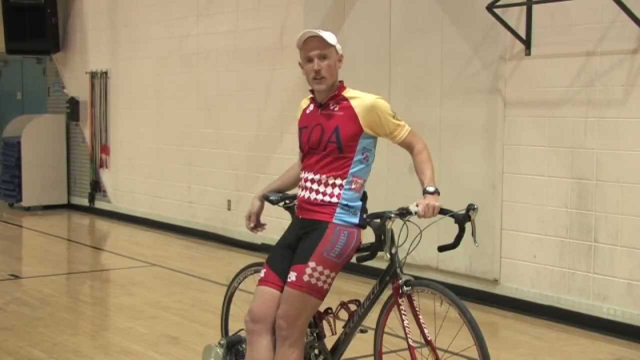 by putting a fist in the middle of your back or gesturing with your hand in a slowing motion. You want to ride in a predictable manner. This is the number one way to be safe and to avoid falls or collisions with other cyclists or motorists.